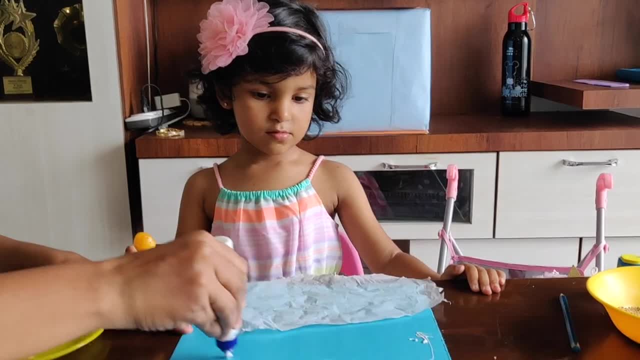 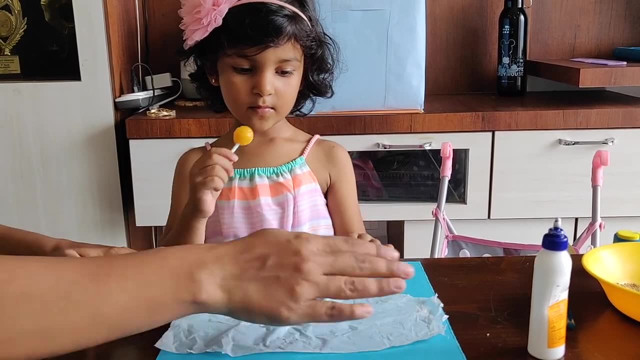 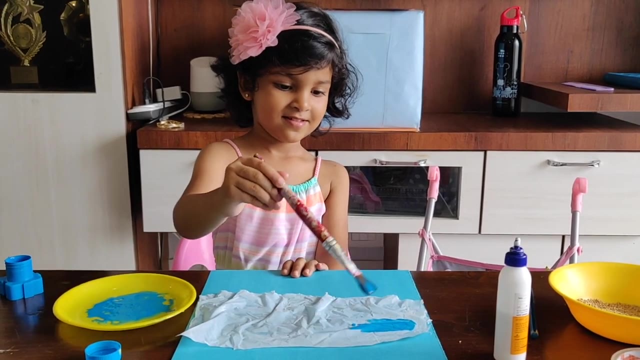 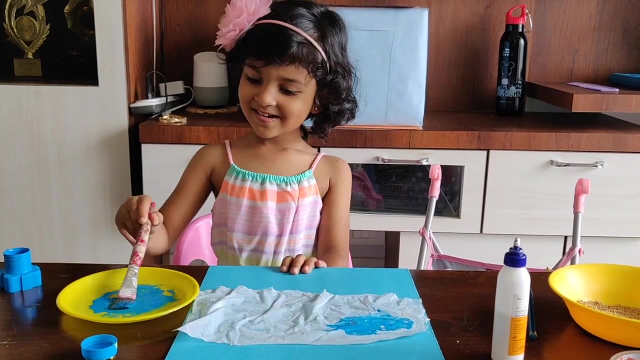 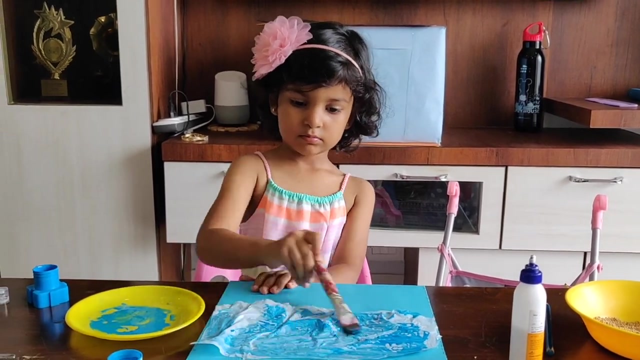 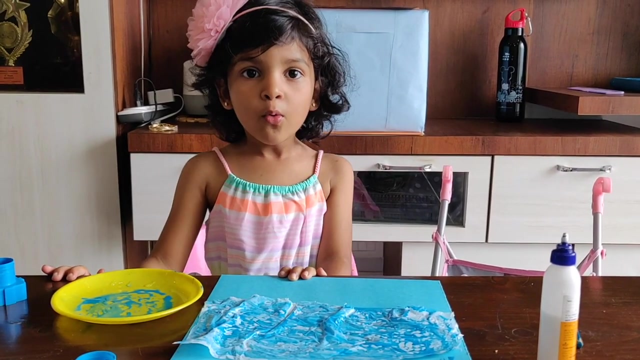 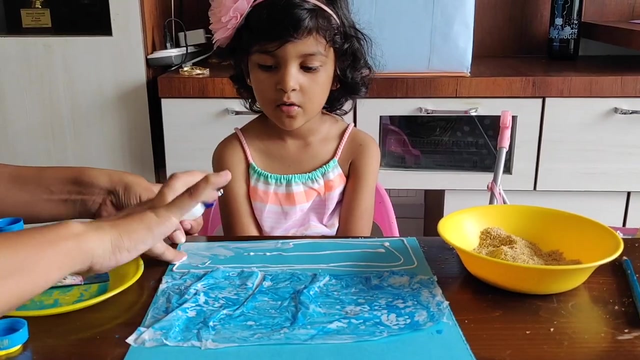 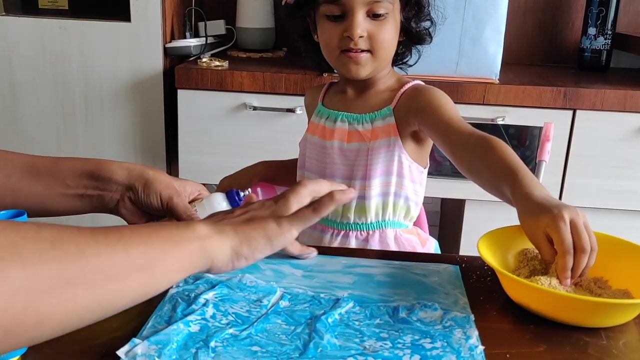 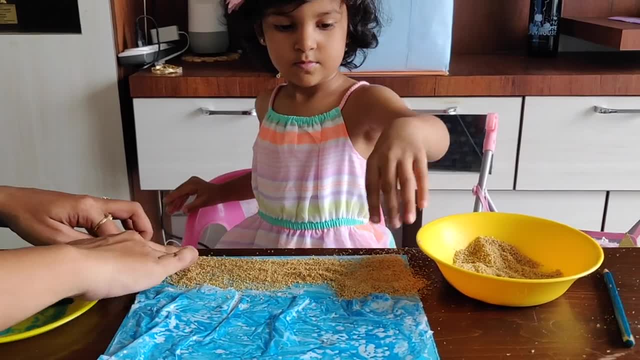 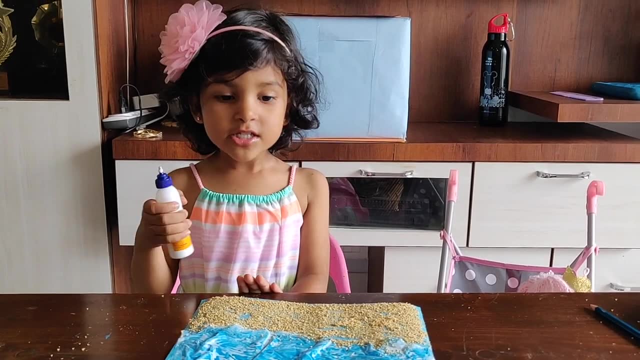 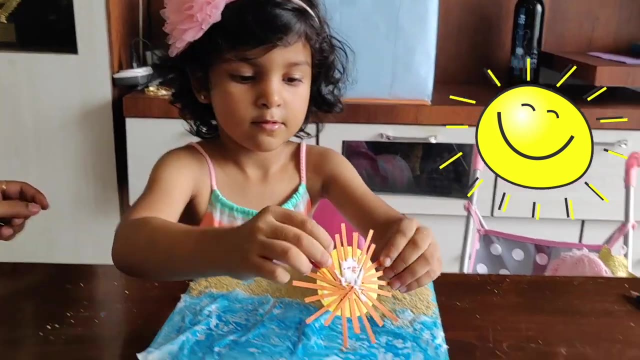 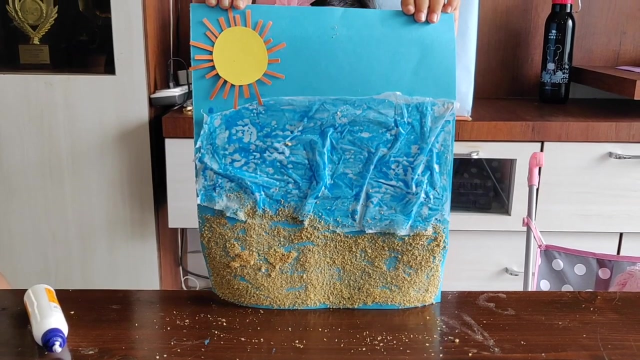 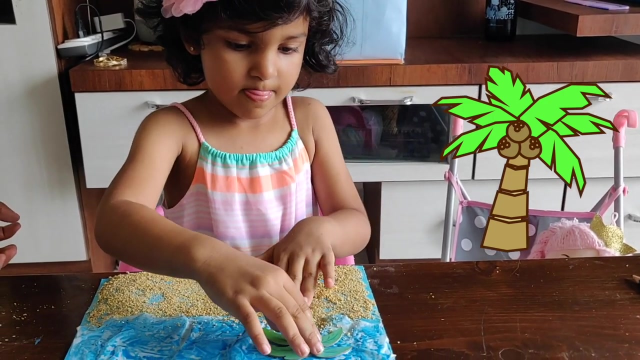 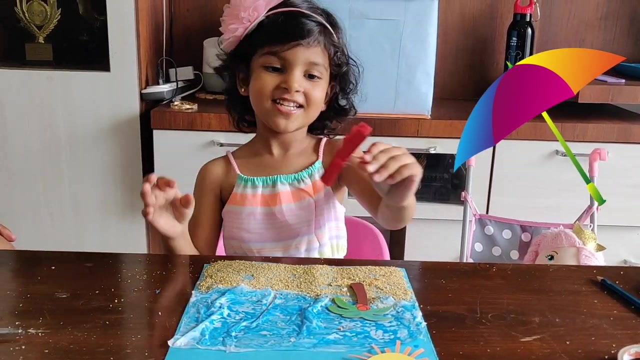 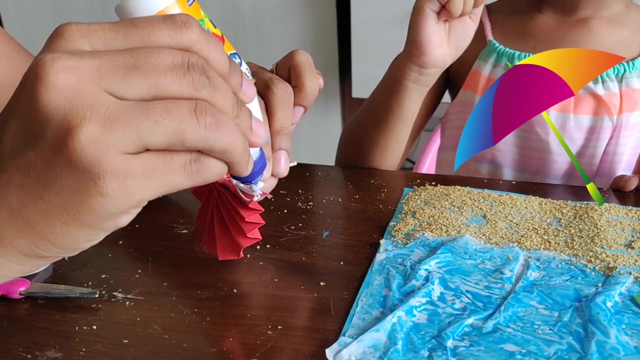 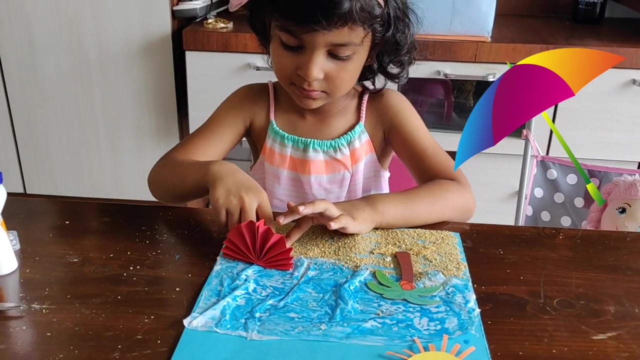 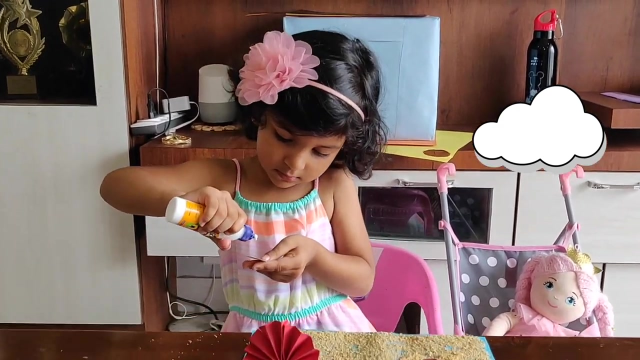 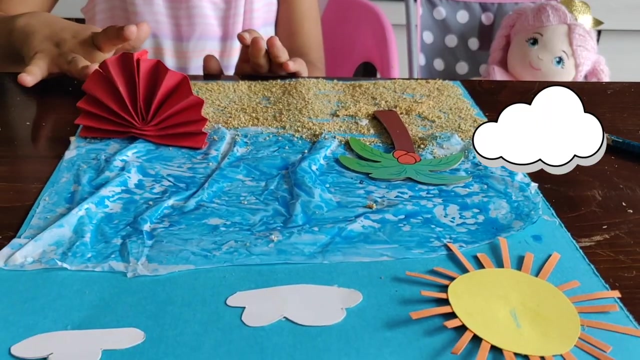 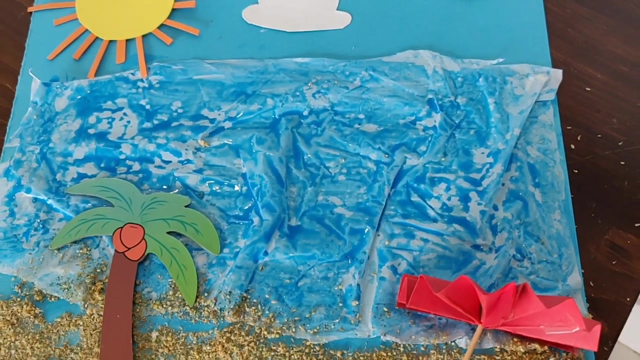 Let's paint the sea water. We are using boxes to mix sand to the sand. We are using boxes to mix sand. We are using boxes to mix sand. Let's paint. Now let's stick the umbrella- See you, umbrella. Now let's stick clouds. 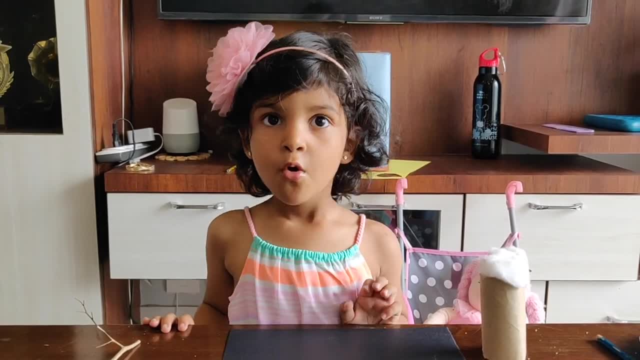 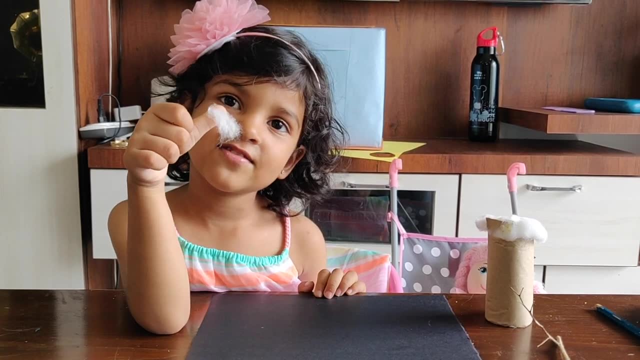 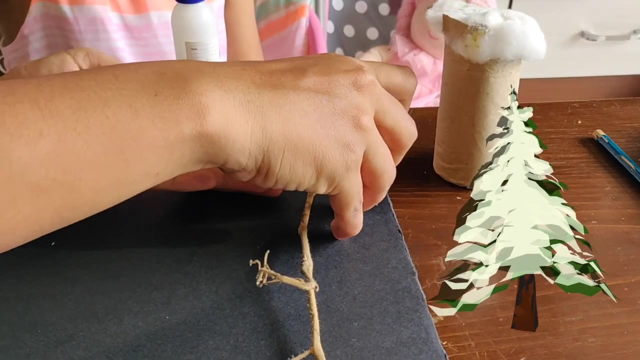 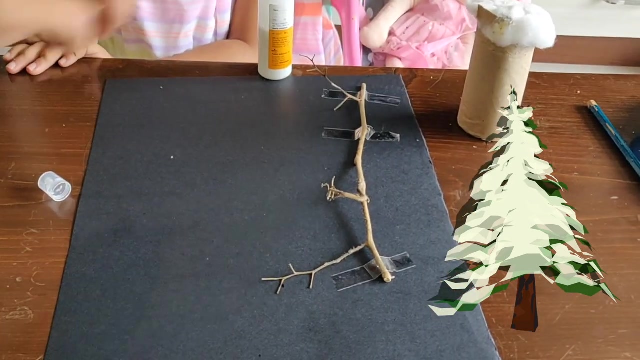 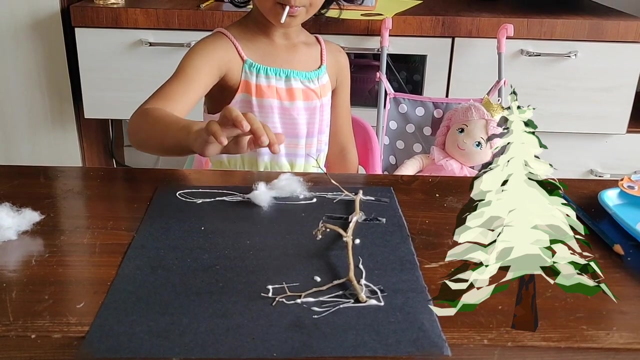 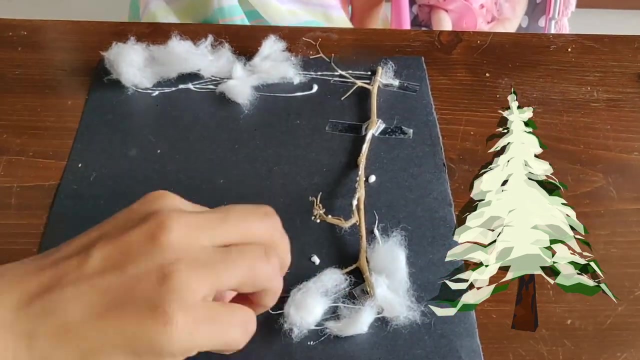 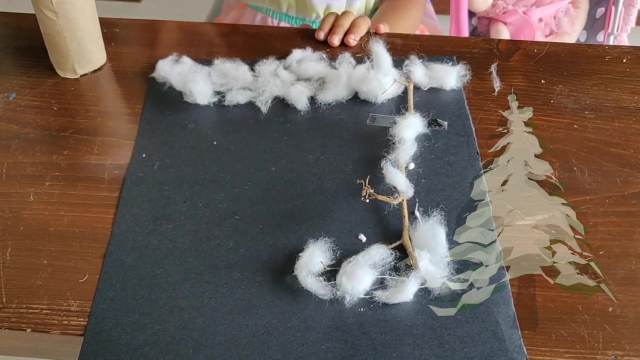 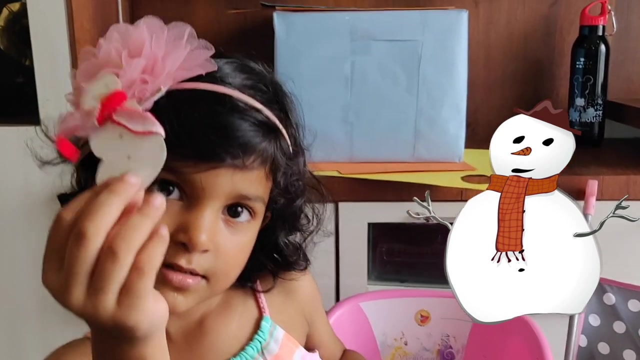 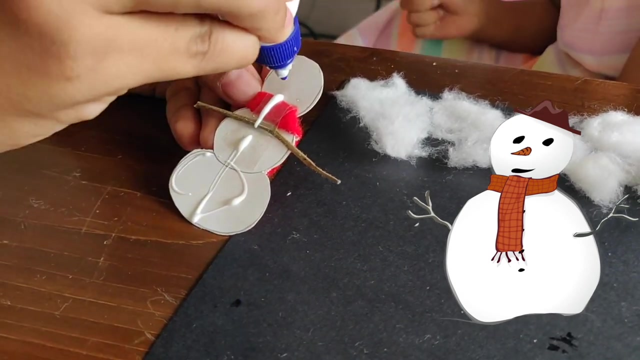 Now we are done with summer. Now let's make winter season. Let's make winter season with this garden. Winter season is for me, and snow. Let's stick the umbrella. We are done. Let's start with flower Smile. Let's make snowman. Now let's stick this snowman. See, It's my cutest moon. Let's stick star in the moon And put a star in moon. And put a star in moon, Don't worry stars. Star in moon, Don't worry stars. 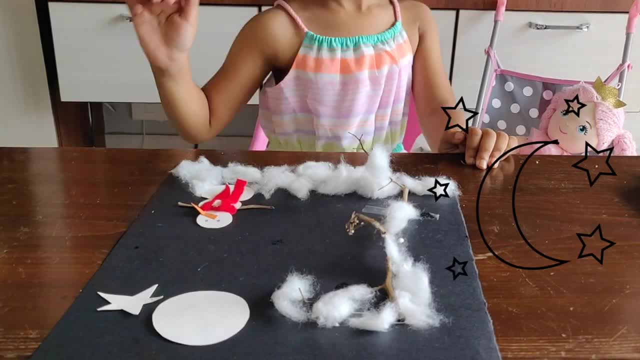 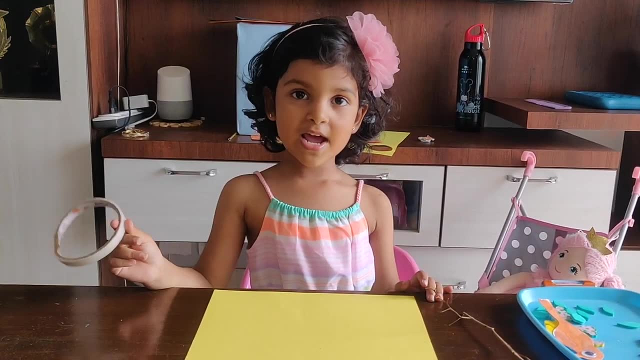 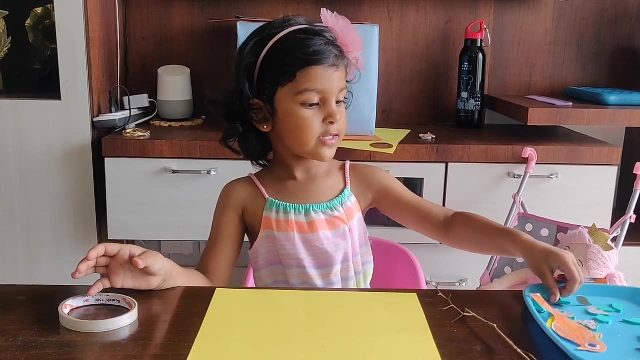 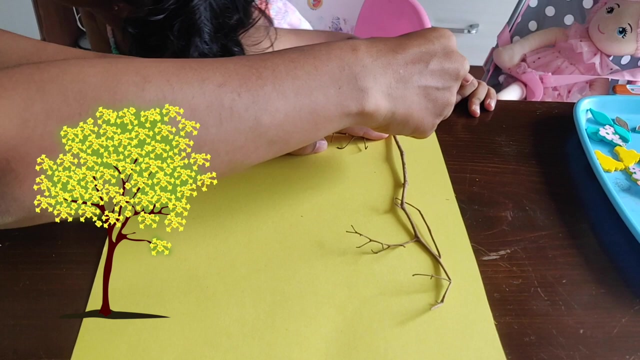 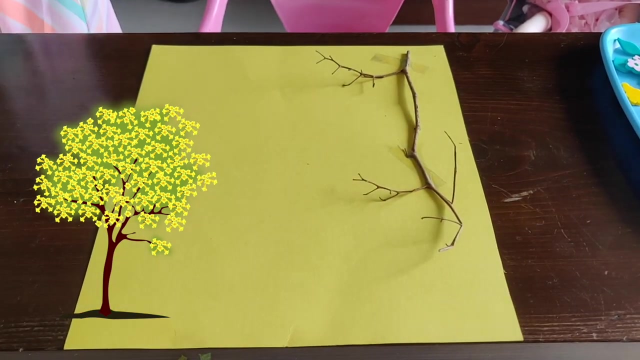 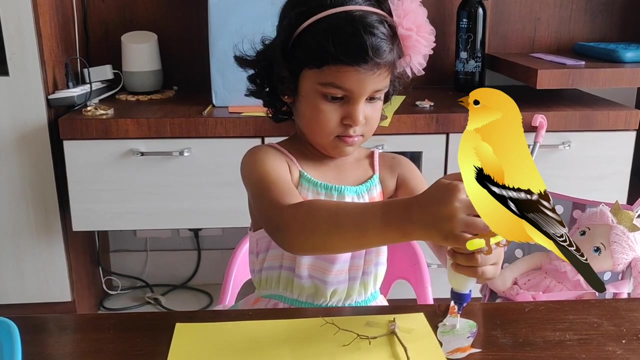 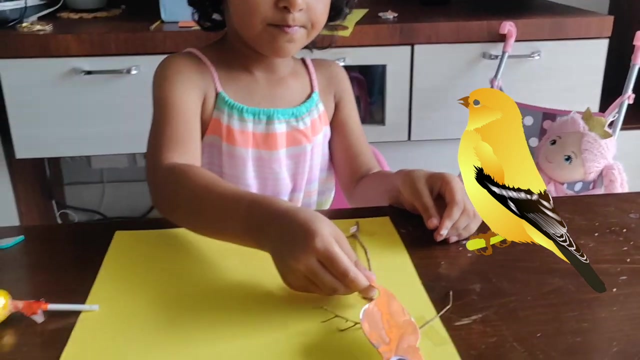 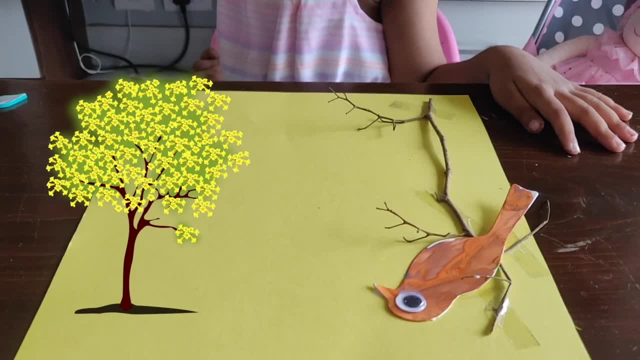 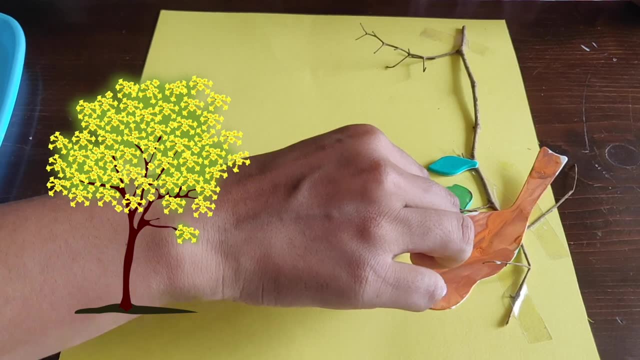 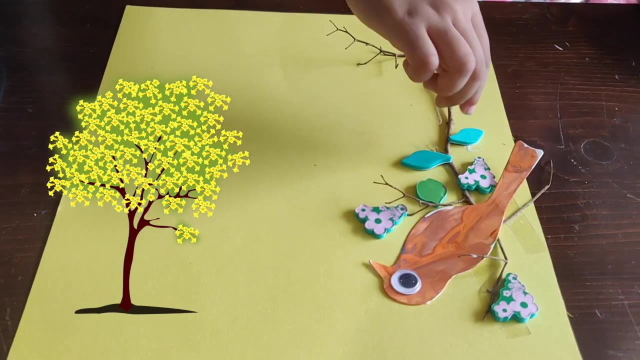 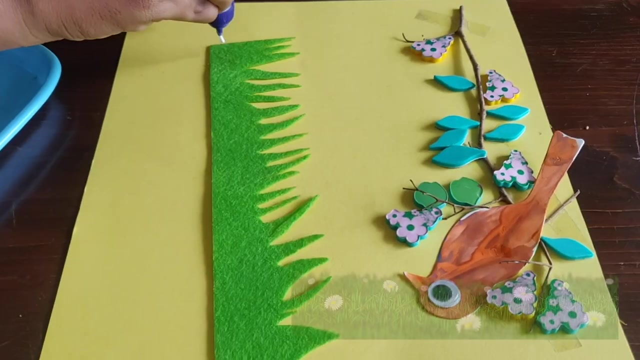 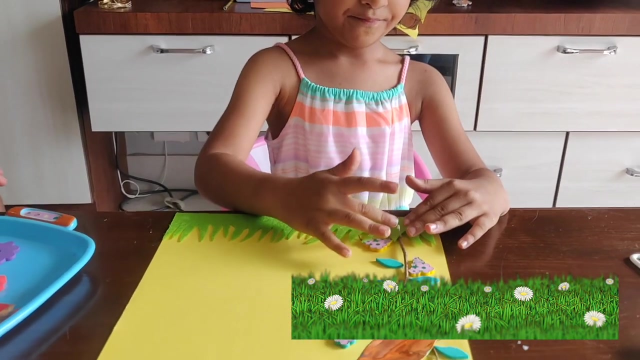